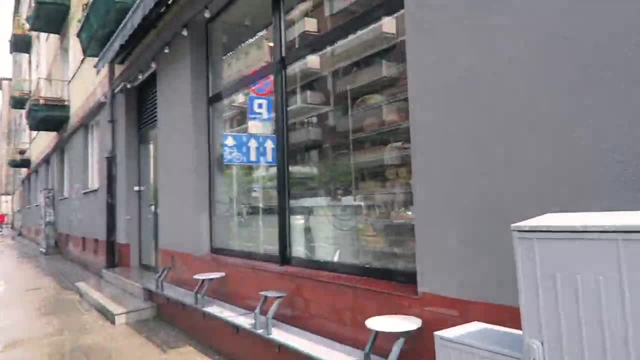 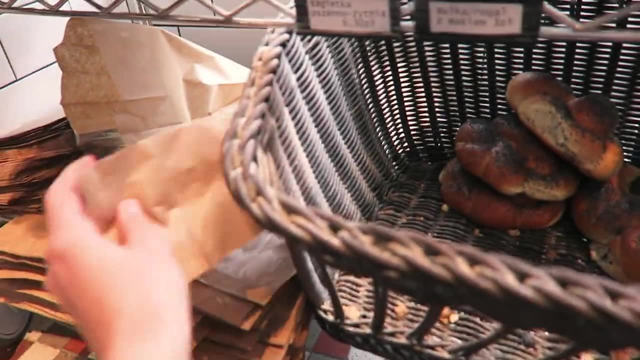 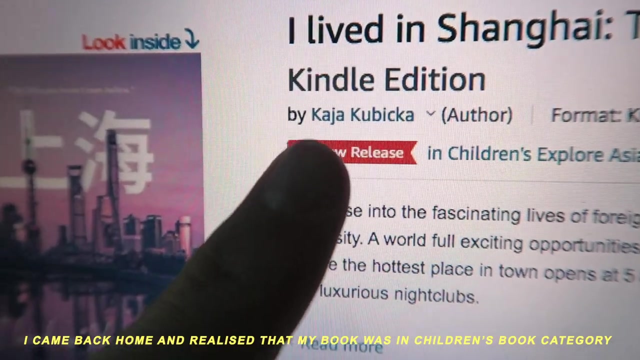 It's this new, or I don't know how new it is, but very nice place. I'm gonna show you. oh, their bread selection is so good. Just look at this. what do I choose? My book is the number one new release. 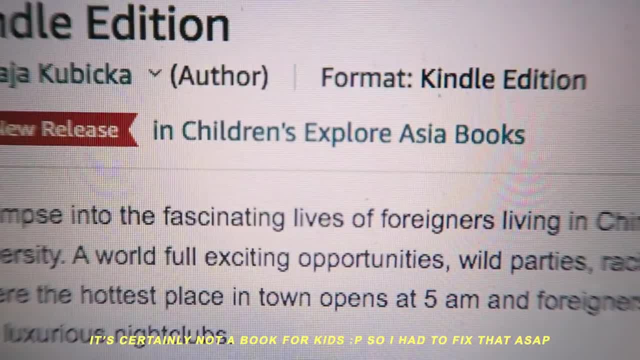 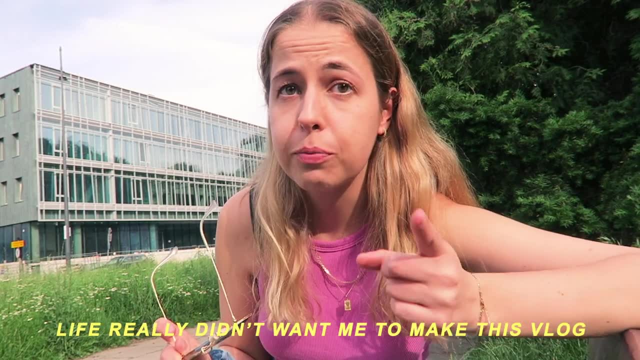 but wait, what's the category? Children's Explore Asia books. that is not good. So unfortunately, vlogging yesterday didn't really work out for me because I had some issues with my book that I had to fix. I noticed that my book was in children's category on Amazon. 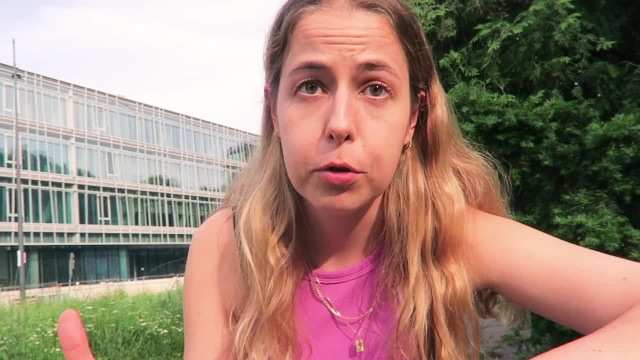 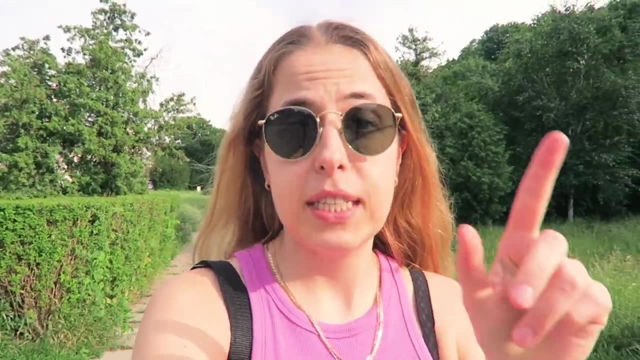 and it's quite problematic because it's certainly not a book for children, So I had to take care of that. Anyway, for now let's get back to Poland. First thing that I wanna say might be a little bold, but I honestly do believe that. 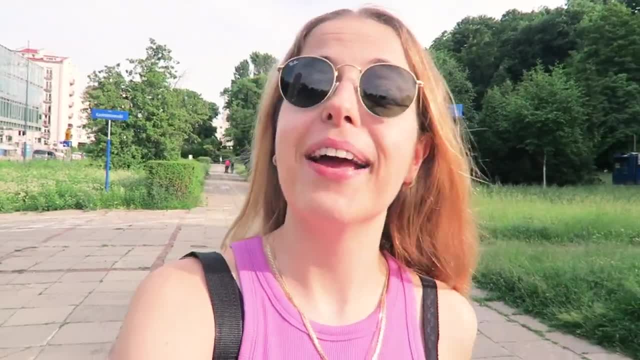 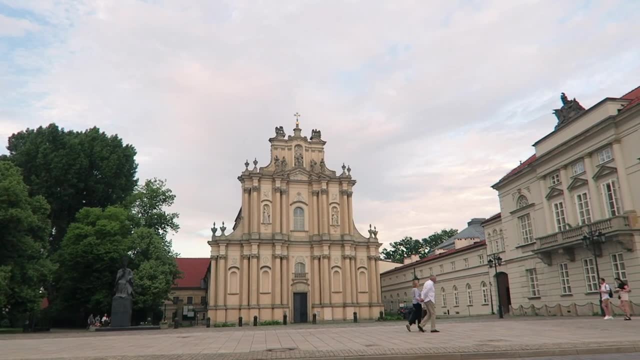 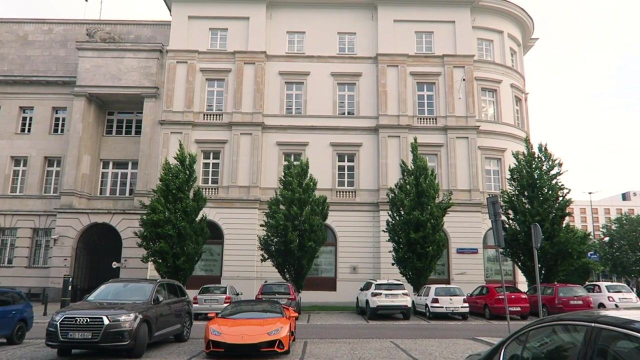 I think that living in Poland is better than many people might think it is. I do think that Poland is one of these countries that is often quite underestimated or people have a very different idea of what Poland actually is. Obviously, there is a good reason for that. 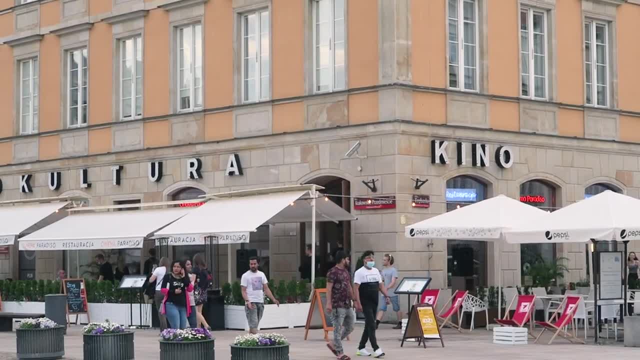 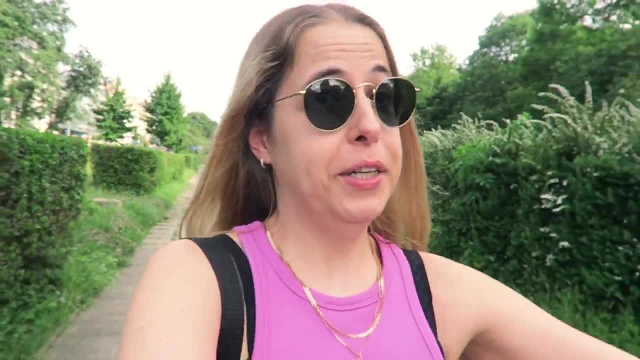 Poland is also one of these countries that just changed a lot and just developed a lot. I think that Poland is one of these countries that just changed a lot during the last couple of years. So if you are someone who visited Poland like 20 years ago or 30 years ago- 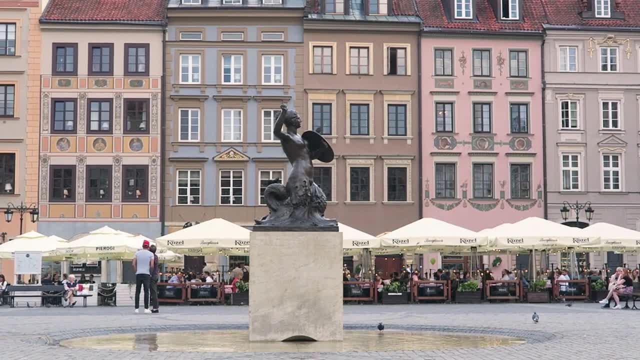 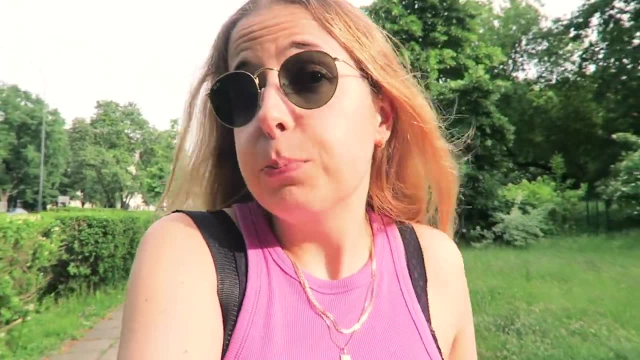 okay, that's a long time, but I would say even 10 years ago, when I grew up, I think Poland was very different to what it is today, And I honestly feel like living here, especially living in big cities, is much better than many people would maybe think it is. 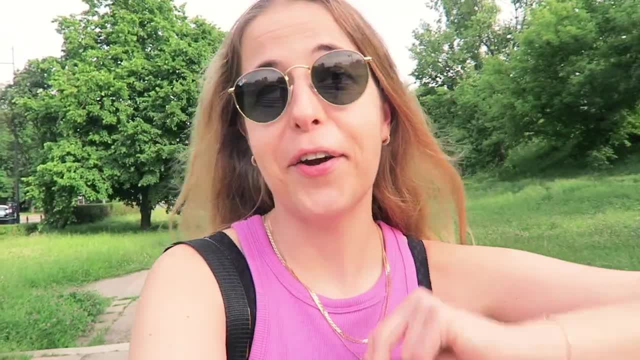 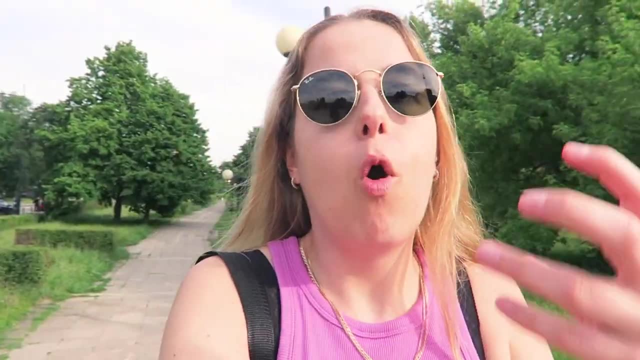 Even the center of Warsaw. this is like the very, very center of Warsaw and it's so green here, And that's the thing about Poland in general- like even big cities are really green, I think Polish cities are very like: livable for people. 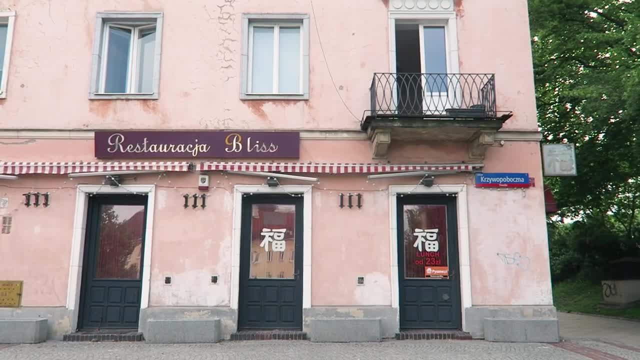 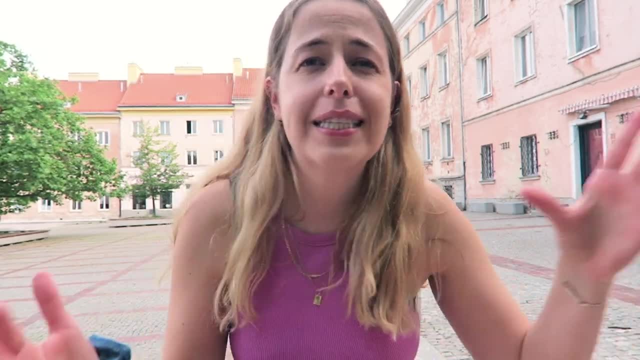 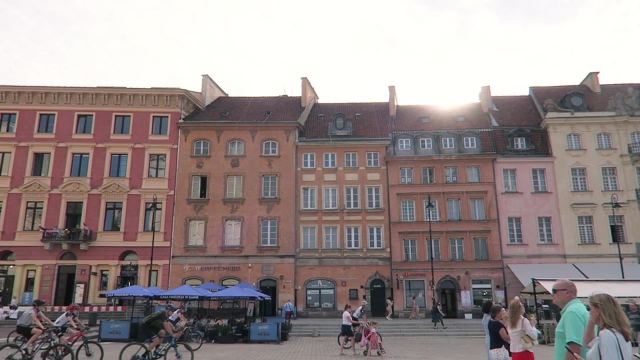 you know what I mean. Poland is a relatively very safe country, And I say relatively because you know like what's safe and what's not safe. it's kind of a difficult topic. The most dangerous city in Poland would probably be Warsaw. 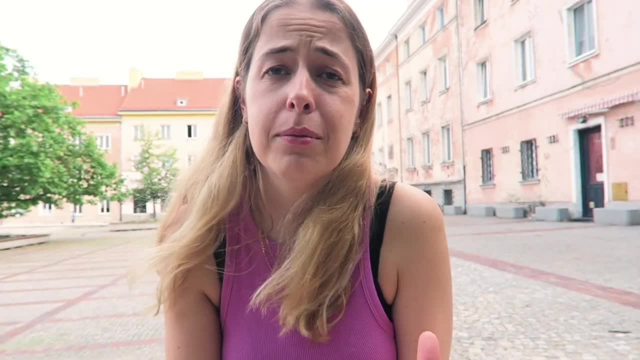 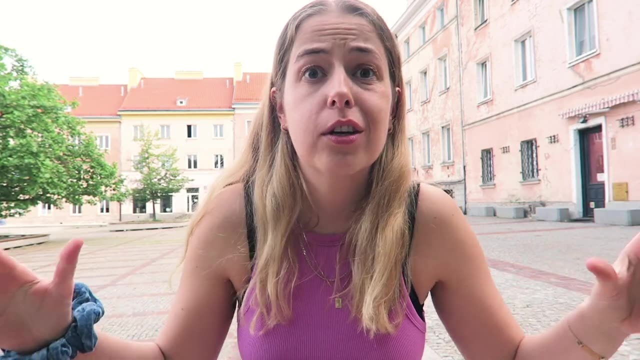 which is where we are right now. The reason why Warsaw is the most dangerous city, it's simply because it's the biggest city in Poland, it's the capital. And I say dangerous because Warsaw is really not dangerous, It's a very safe city. I would say. 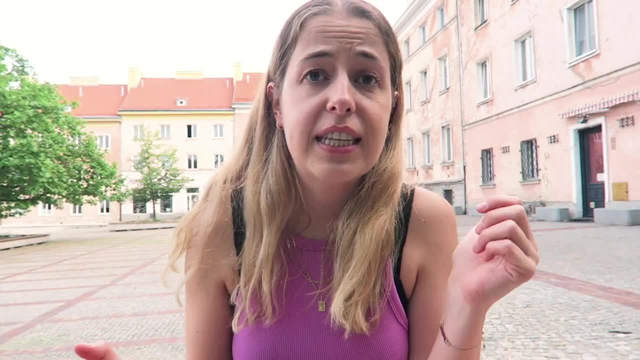 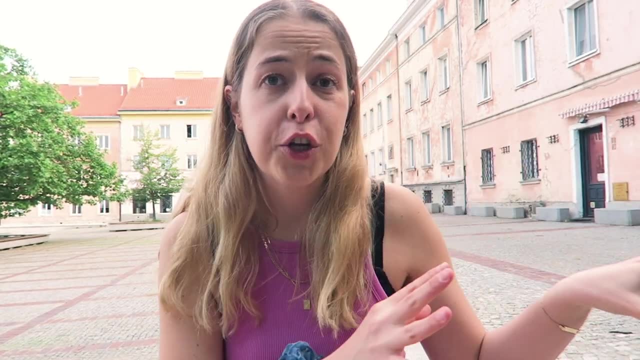 I feel very safe and comfortable here. I would say that Warsaw is definitely much safer than any city in the US and probably much safer than majority of Western European cities. I'm probably gonna refer to US a lot in this video because I know that a lot of people 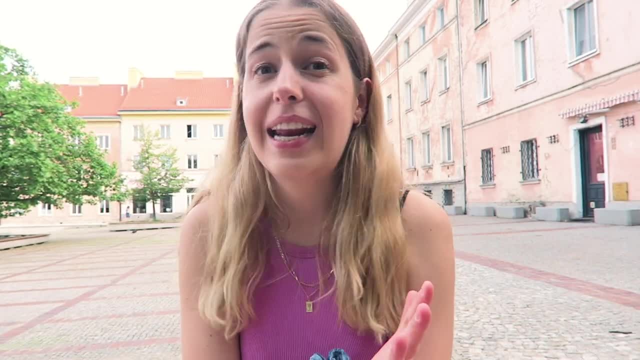 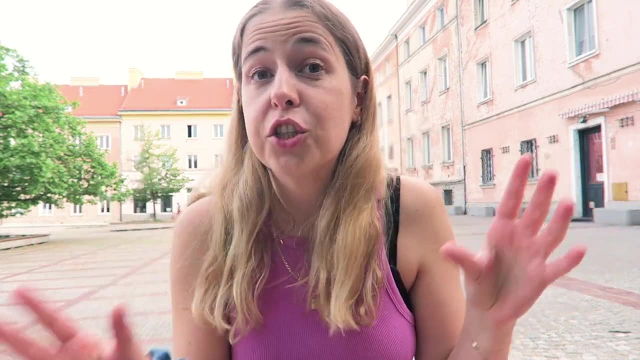 that tend to watch these videos about Poland are from the US, and I assume a lot of you guys- or I see from the comment section- that there are also quite a lot of people who are second generation Polish people born in the US and they're often interested in this type of videos. 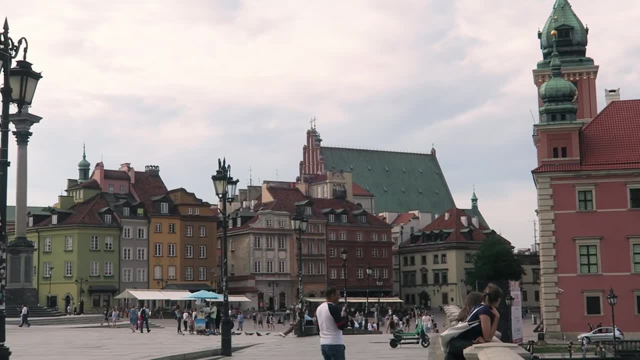 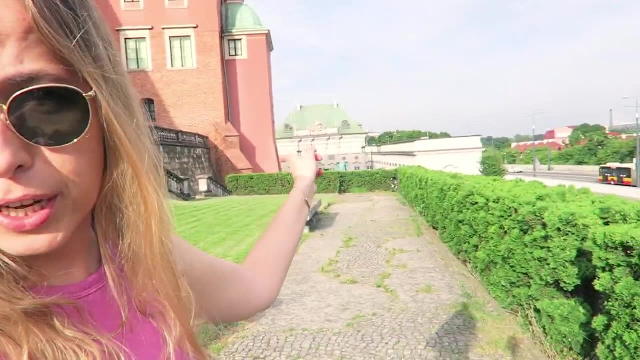 This place right behind me is the castle square. This is the center of Poland. This is the center of Poland. This is the old town in Warsaw. I am attempting to make it to this pretty building right there, because I always look at this building and it's so pretty. 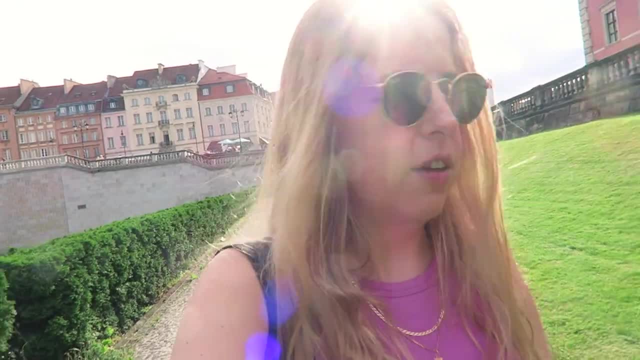 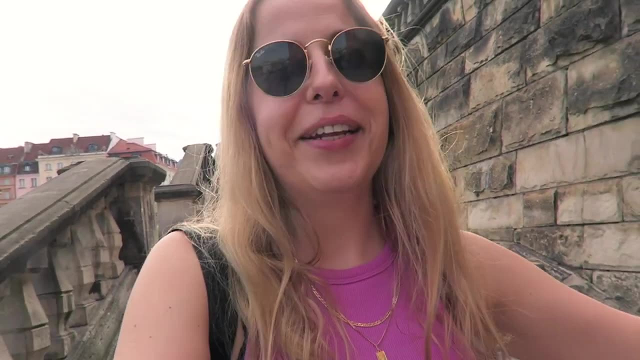 but I just I never go there. Not that there's anything to do there, I think. but let's see, In Poland we do pay taxes. I mean, do pay taxes? Obviously we pay taxes, but the taxes here are kind of like European standard taxes. 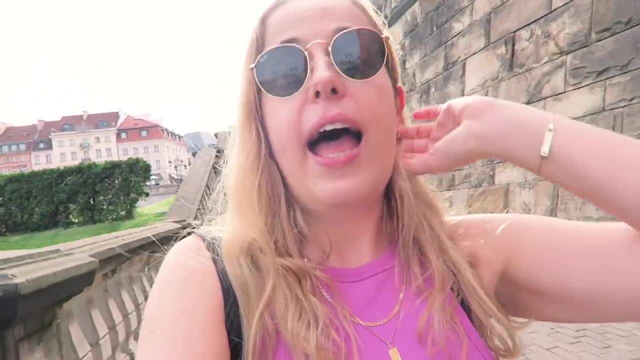 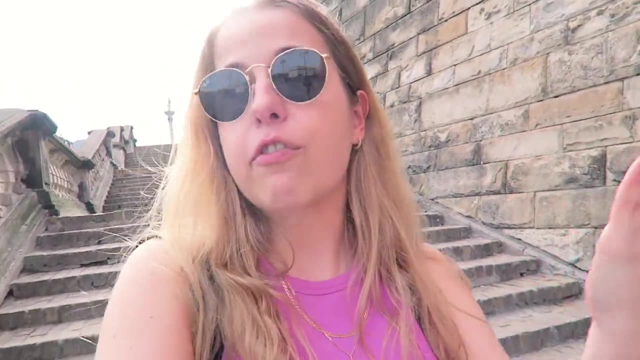 They're much higher than what you pay in the US, for example, and because of that, we have public healthcare, We have public education, Schools are free. Of course, we have private schools in Poland as well, And often the private schools are considered better. 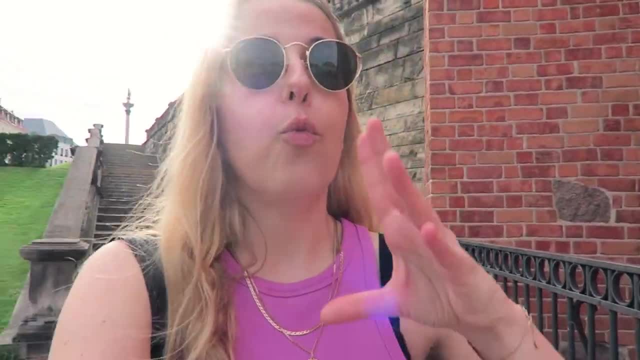 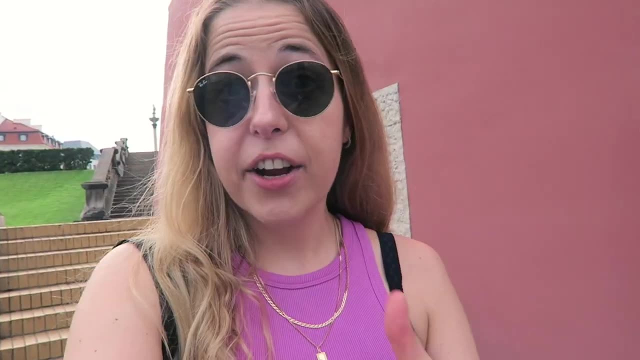 but it's definitely not like in some countries where if you want your kid to go to a good school, then you need to put them in a private school. This is not the way it is here in Poland. Higher education is free, meaning university is free in Poland. 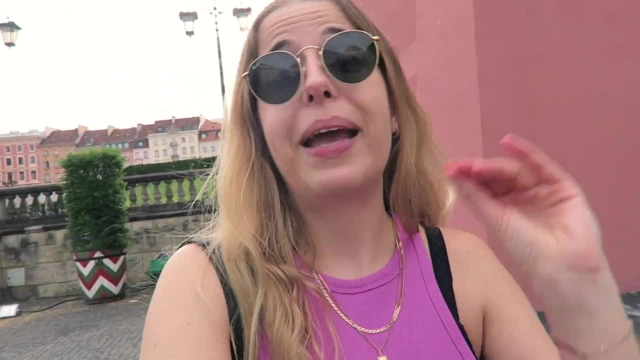 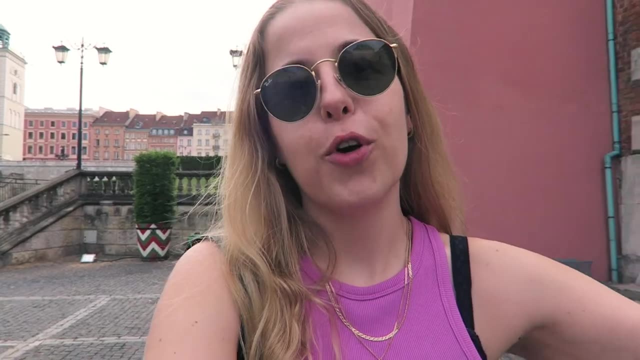 When I said that in one of my videos, some people corrected me that it's not free because we pay taxes for it. And yes, I completely agree with you. It's not free in that way, because we all pay taxes for it. Of course, nothing falls from heaven. 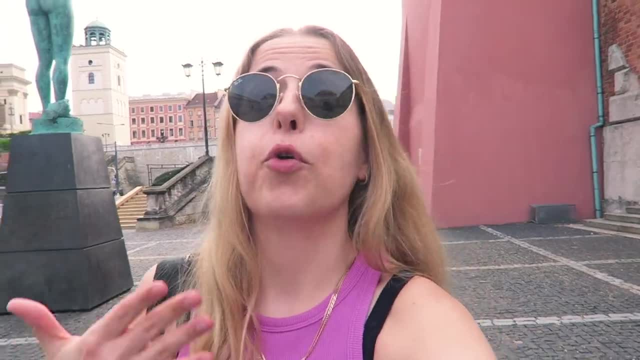 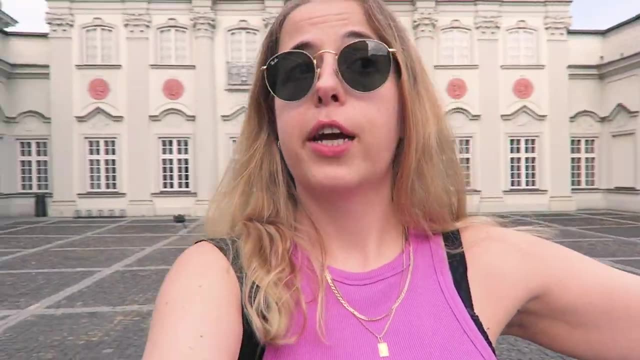 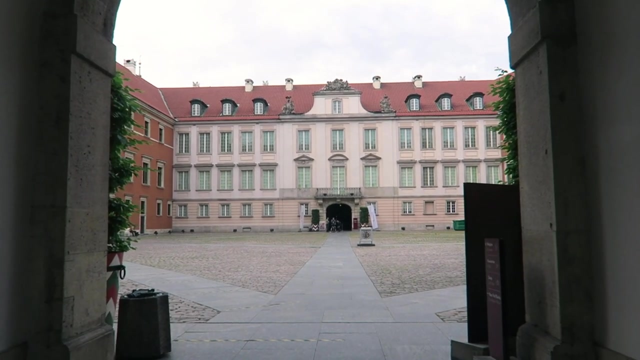 but when you want to do a university degree in Poland, you don't pay because it's paid by taxpayers. So, as you can see, we made it to this pretty building that I was trying to make it to. It is very pretty. So this is the inside of the castle square. 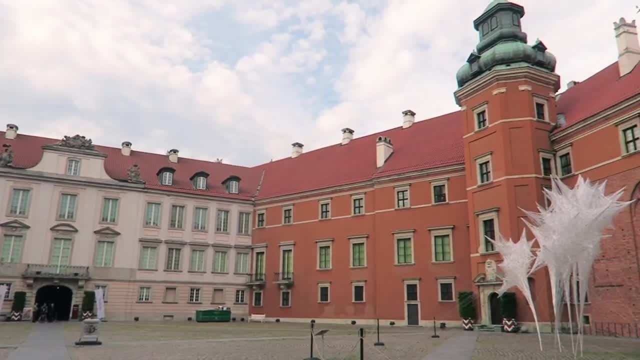 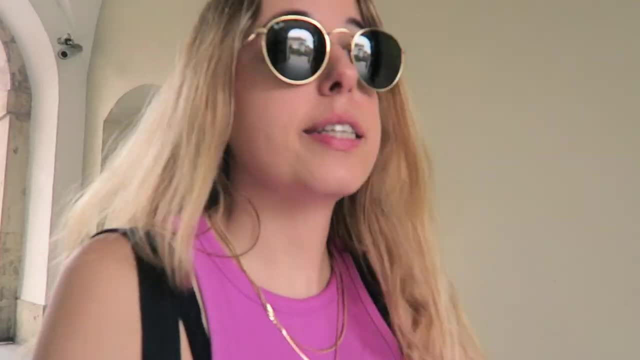 castle square of the castle. So you obviously do need a ticket to see it. So that's not something we're going to do right now, but good time seeing the inside. And also something that I keep thinking is that this church is massive. 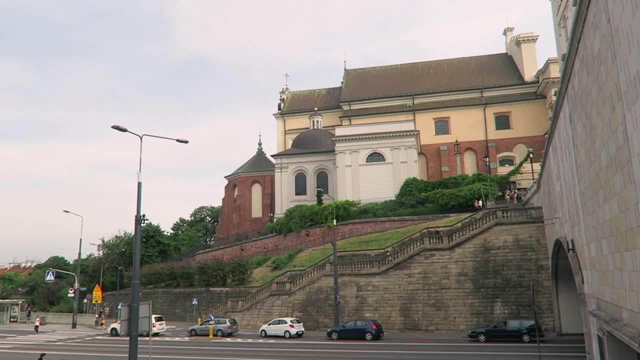 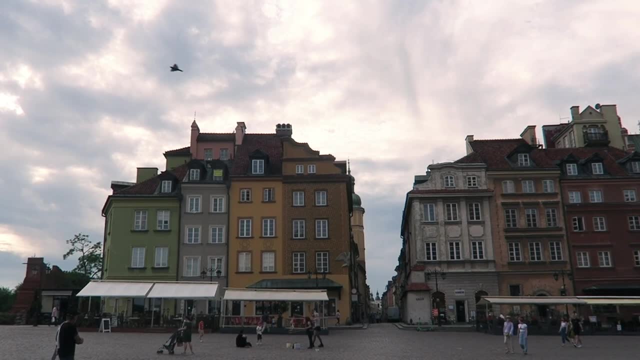 One thing that you obviously must know about Poland is that we do have a lot of churches here, So majority of Poland's population is Catholic, So there are a lot of churches. It is unfortunately a little gloomy today, which is a bummer, because I really hope to film this video. 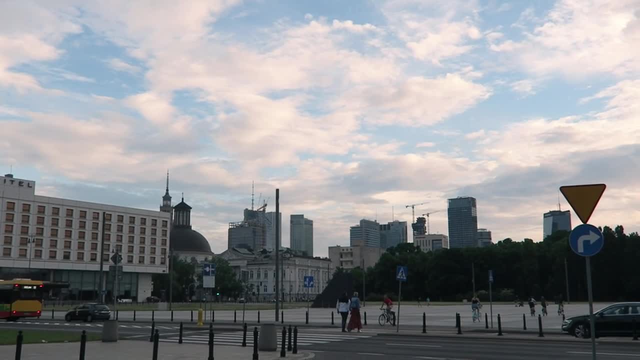 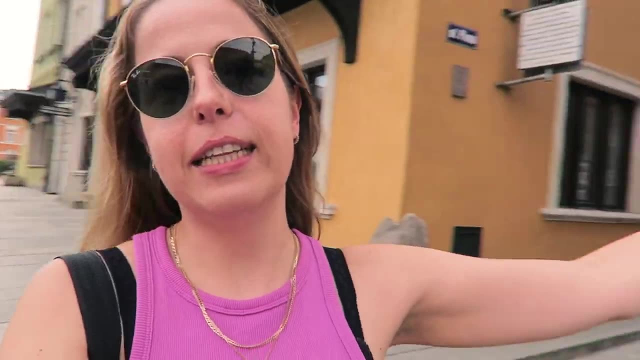 when it's sunny outside. Unfortunately, as much as I love Warsaw, Warsaw is a very gray city. Maybe not here, Like right now. we're in the old town And, like, as you can see, the buildings are very colorful here. 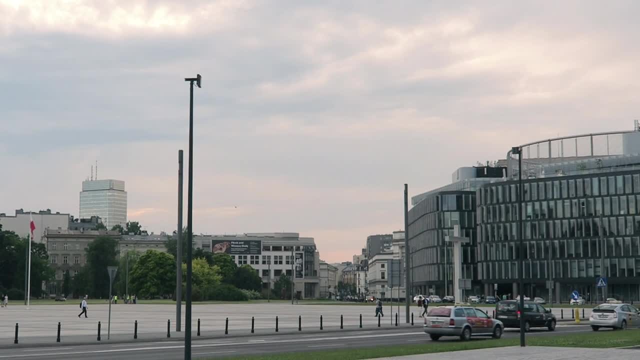 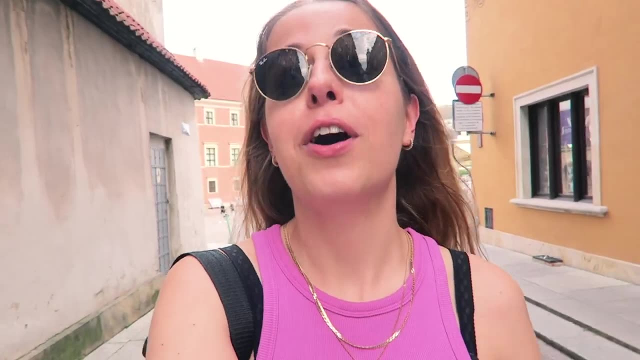 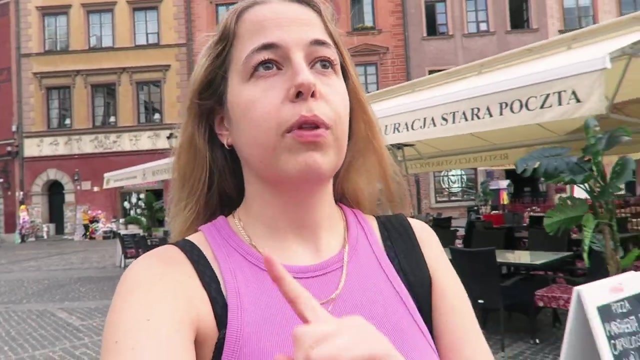 But in general in the rest of the city, like there is a lot of gray. So when the weather is bad, which is unfortunately quite, I mean the weather is bad a lot here, So the city just looks very gray. So the place where we are right now, 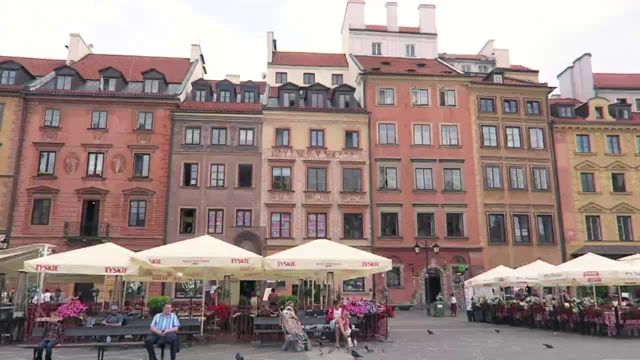 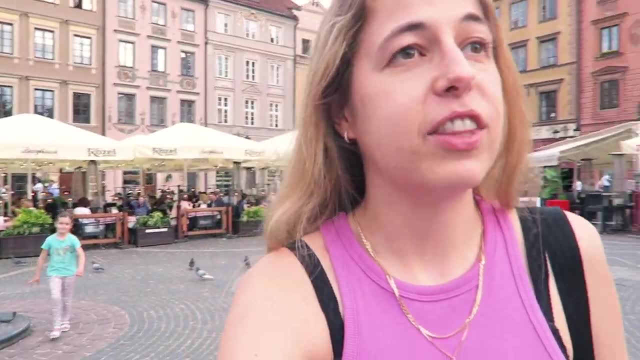 it's called Market Square. I come here sometimes, too, for dinner. It's really nice, especially in the evening. I mean, as you can see, it's super beautiful, So it's a nice place to sit and have dinner, Something that I think is like one of the best things. 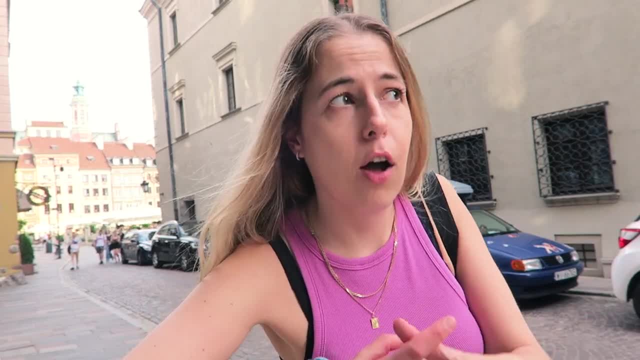 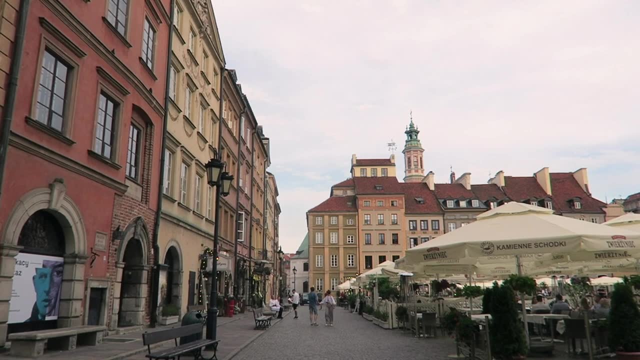 about living in Poland is the fact that the country has a very long and rich culture and history, And obviously that makes it really interesting to live in a place like that. There are a lot of nice places in Poland where you can travel, both like interesting cities. 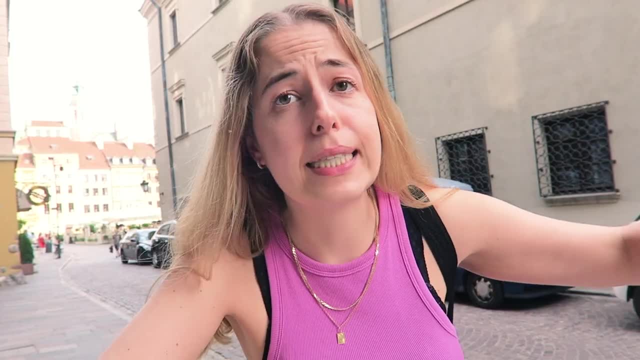 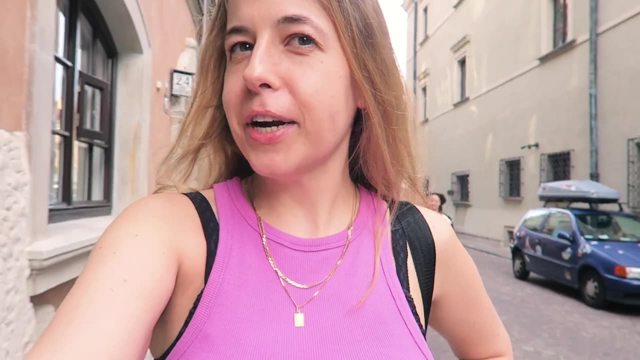 but also, like nature wise, we have mountains, we have lakes, sea, So I thought I will mention that. But anyways, okay, let's move on to the more negative sides of living in Poland. I guess that you should definitely know. 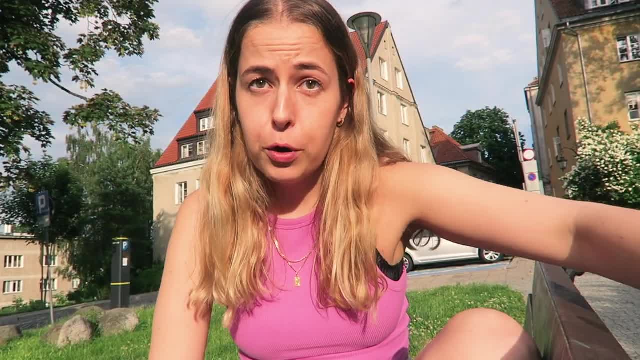 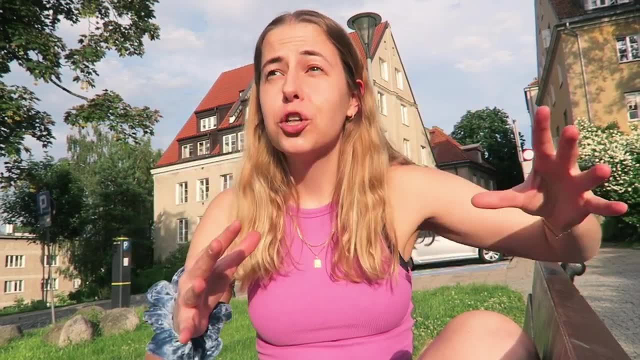 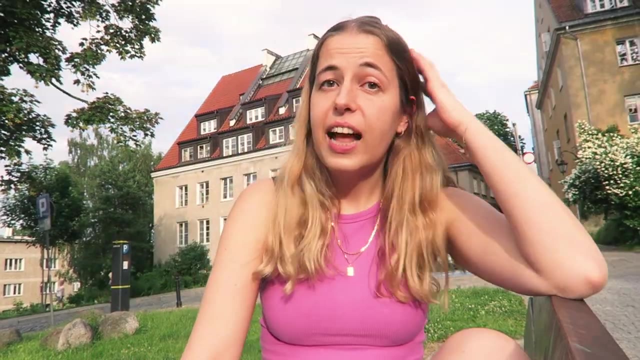 So the worst thing about living in Poland, and something that you should definitely know if you're considering to move here, is the fact that wages- salaries, are still relatively low here, Much lower than in other Western countries, much lower than in Western Europe or in the US, obviously. 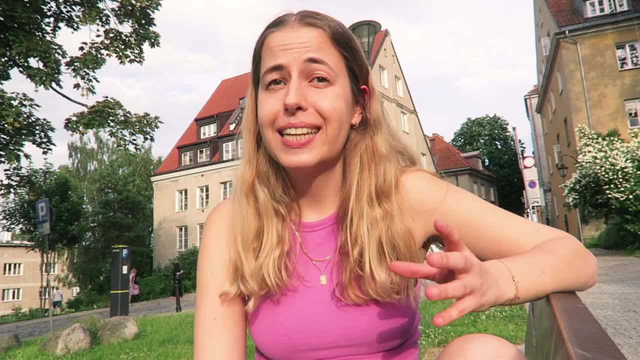 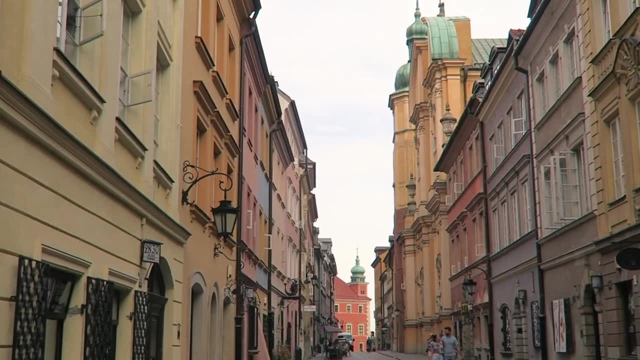 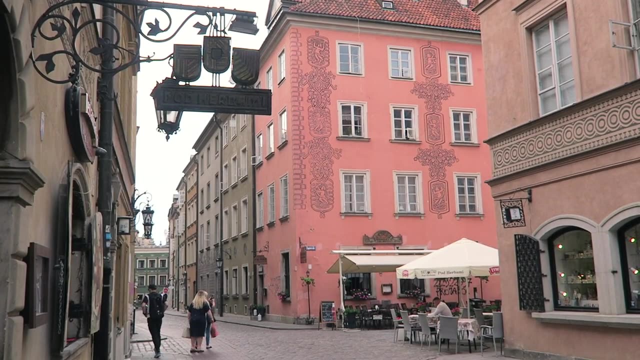 That's, of course, really annoying and upsetting, And I really hope that this is something that will change in Poland. It is slowly changing, but I mean slowly, And what's kind of happening here right now is also that inequalities in societies become bigger and bigger. 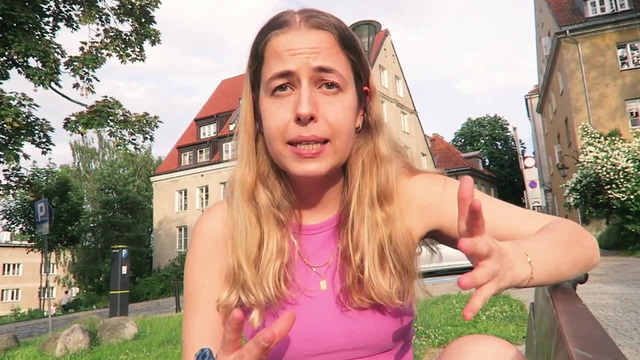 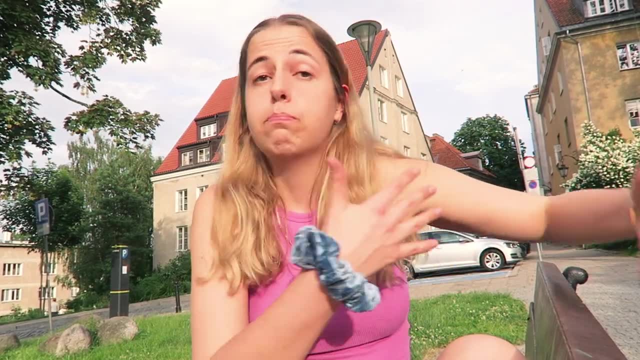 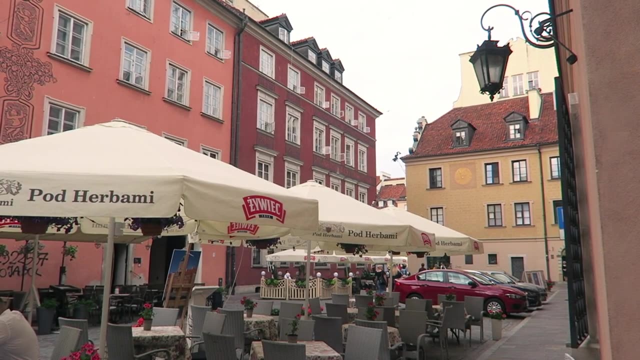 The thing is that some people in Poland, especially in big cities, are already starting to earn wages that are very similar to Western countries or the same as in Western countries, But then there are still some people who earn salaries that are much lower, and that creates a lot of inequality in the society. 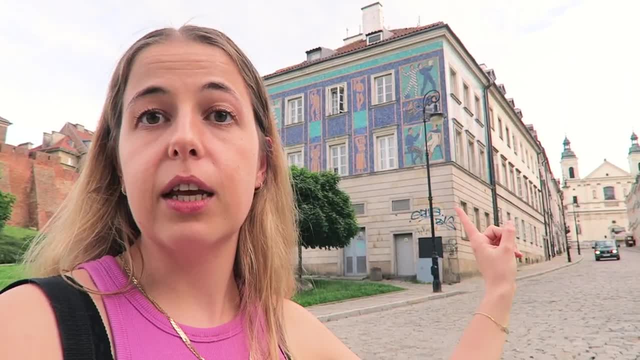 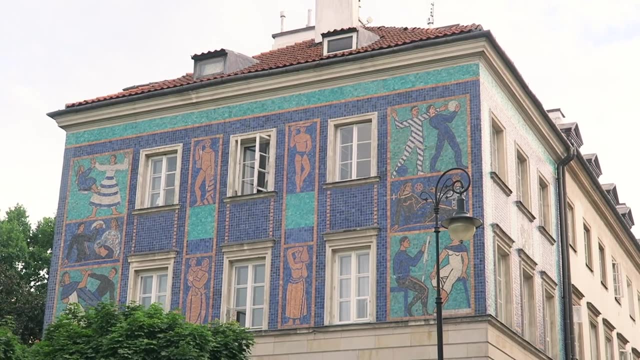 Another thing to mention is that this is like one of my favorite buildings in Warsaw. How pretty is it right? In general, this street is just really pretty. I'm sure there are a lot of people who would like to have options to explore here, obviously like 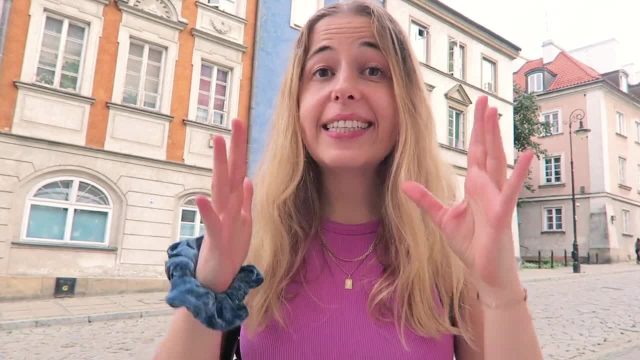 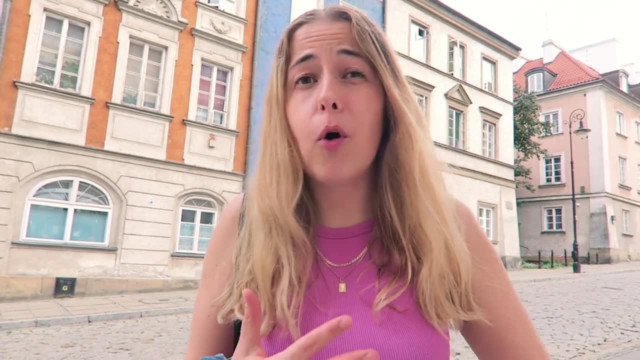 How are they going to manage that route? I would say it is really, really an interesting city. It's usually very different. Another thing that you might be interested in is: how does it work when it comes to finding a job when you are a foreigner? 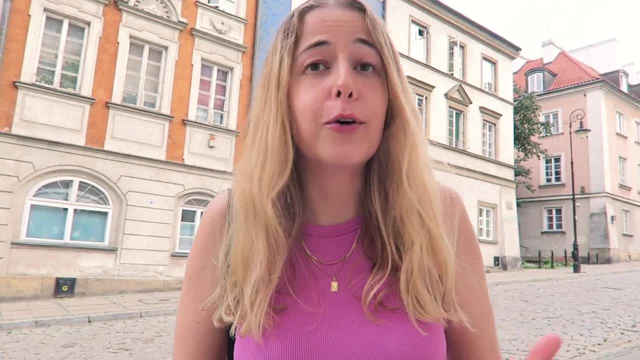 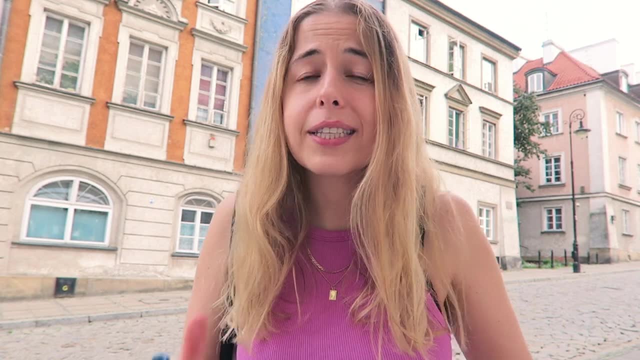 especially if you don't speak Polish. Obviously, I'm not going to say that finding a job in Poland when you don't speak Polish is super easy, because, well, Polish is the official language here and it is the language that we all use and speak. 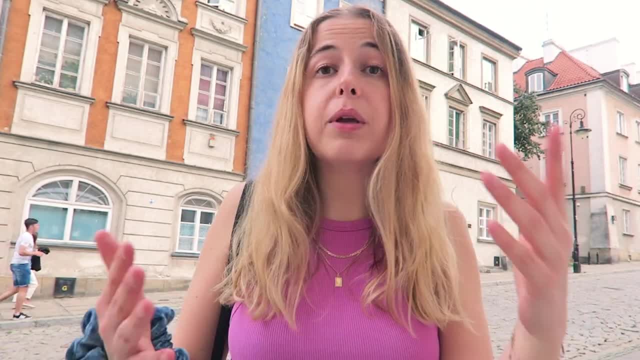 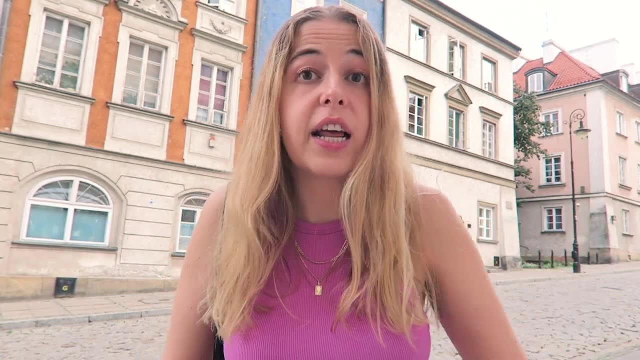 Krakow and the company where I used to work, there were quite a few people who didn't speak Polish at all, and since the language that we use on the daily basis was English, it was not an issue like at all, so it is definitely possible to find. 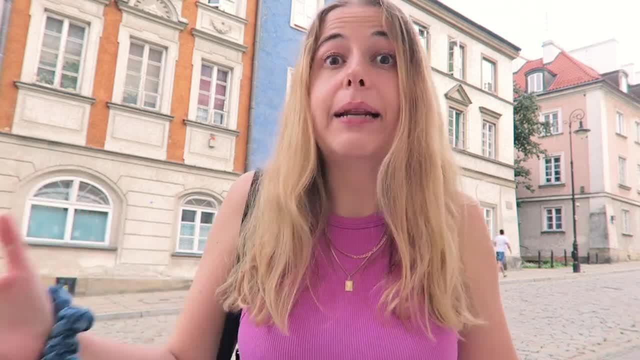 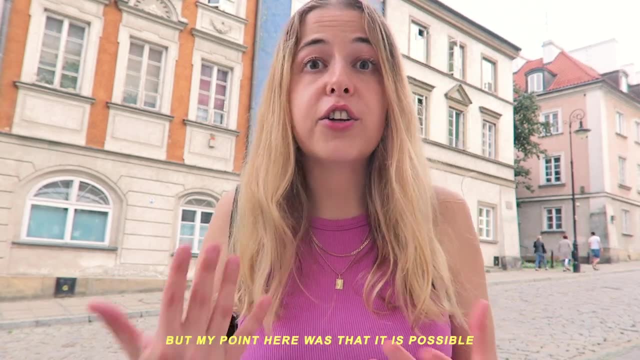 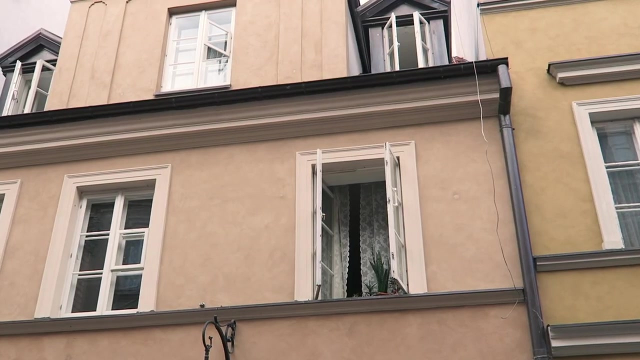 a job here if you don't speak Polish? yes, that it might be a little bit more challenging in general, but in big cities, especially here in Warsaw, there definitely a lot of international companies who use English on as their- you know- first language. what is the attitude of Polish people towards? 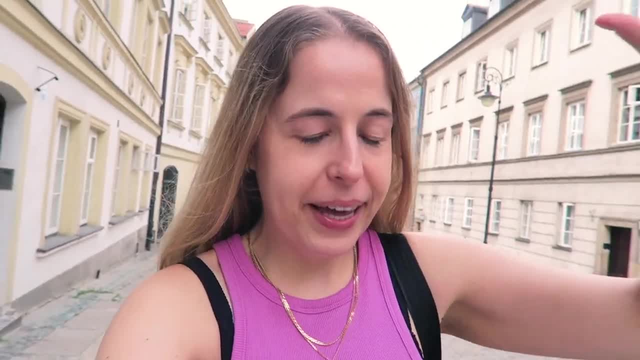 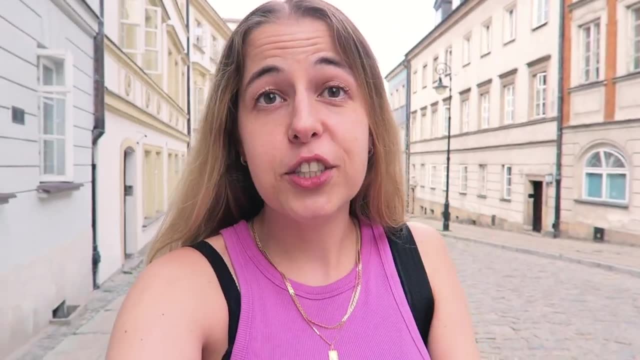 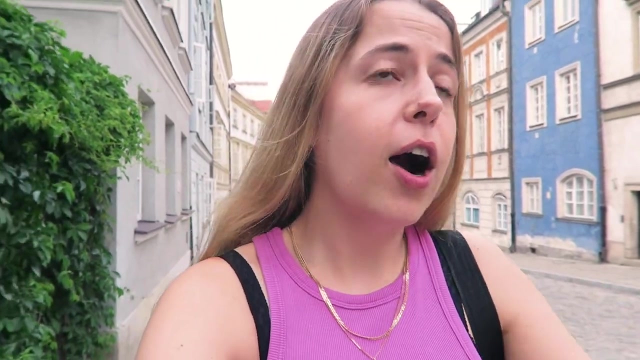 foreigners. this is again a very, very deep topic. I would say in general, it's pretty good. I would say, in general, Polish people are quite curious of foreigners and they like always love to know what foreigners think about Poland, and I would say that in general people are quite welcoming. however, I also do 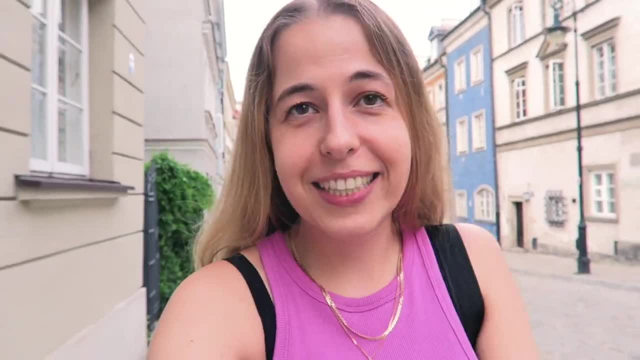 understand that Polish people are very welcoming and I would say that, in general, people are quite welcoming. however, I also do understand that I'm certainly not the best person to ask this question, because well I am. I'm certainly not the best person to ask this question because well I am. 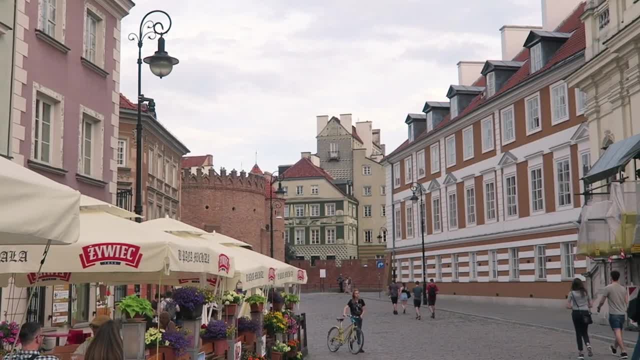 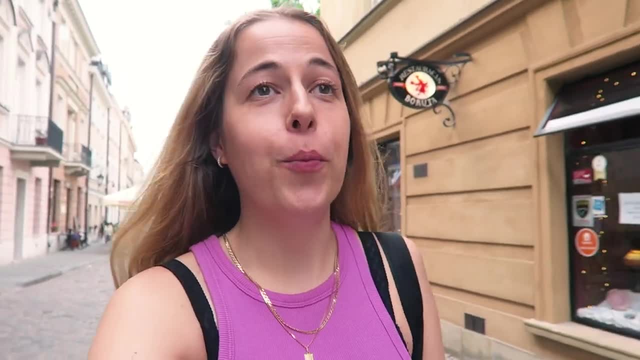 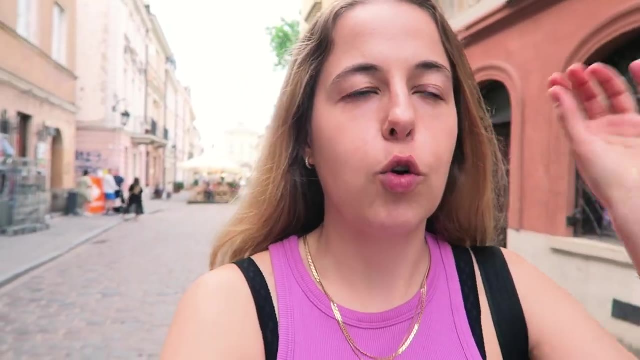 Polish. I speak Polish, getting really tired so I think I'm gonna head home. whenever I walk around and vlog, I really get like extremely tired. I think it's because, like, vlogging really requires my brain to work and it's like highest level. so I'm 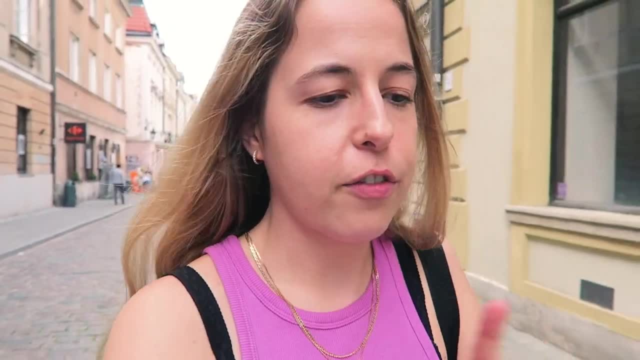 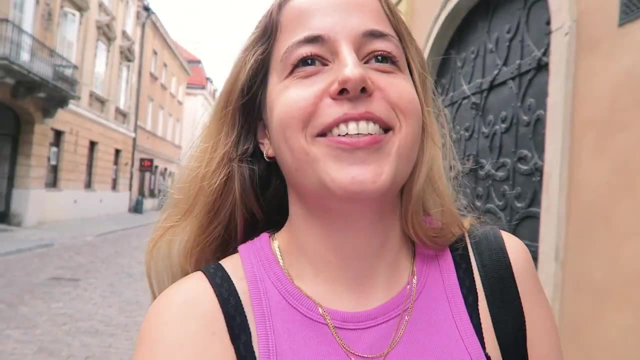 gonna head home now at at home, I'm gonna mention a couple of. I am going to mention a couple of things that I want to mention about finding an apartment in Poland and like things that you should keep in mind. I feel like things you should keep in mind. 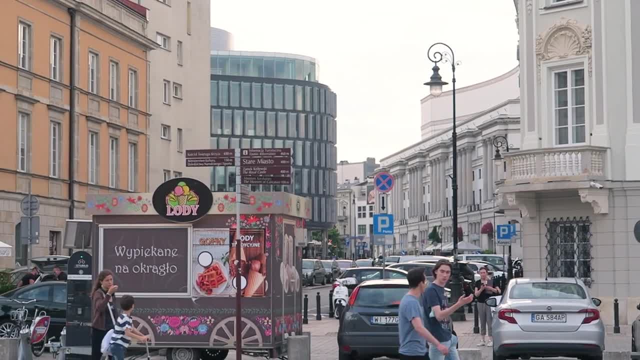 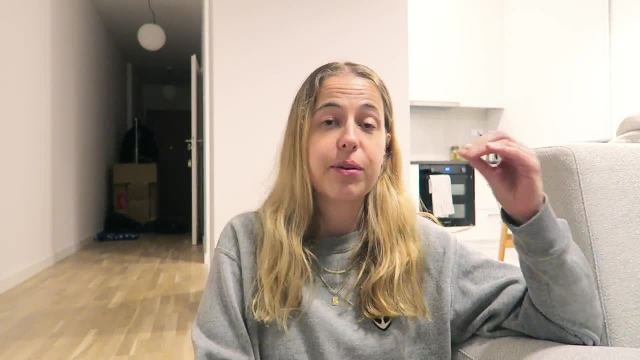 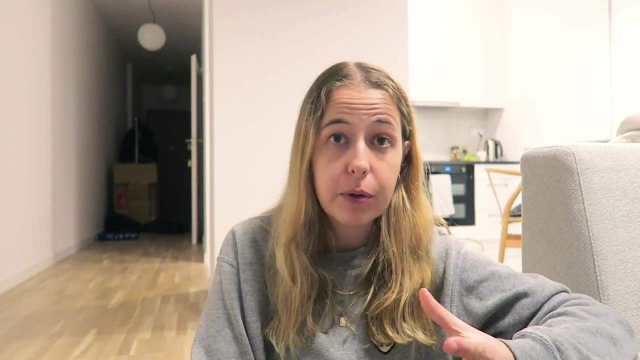 is like a sentence that repeated at least like hundred times in this video. in general, I would say that it's surprisingly easy to find a place to live in Poland or Warsaw. that's where I live, and the reason why I say very easy is because a lot of people who have you know lived in big cities like Paris. 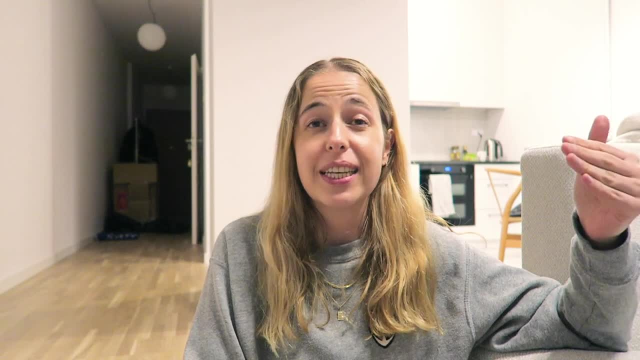 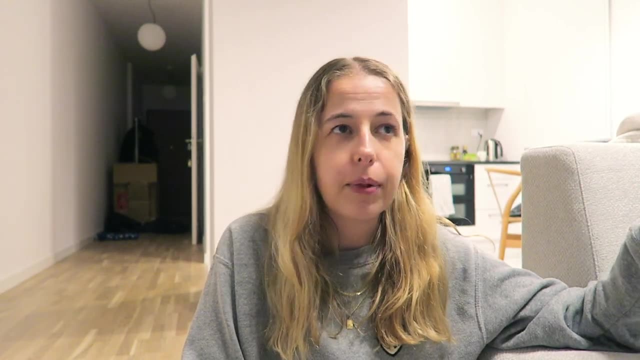 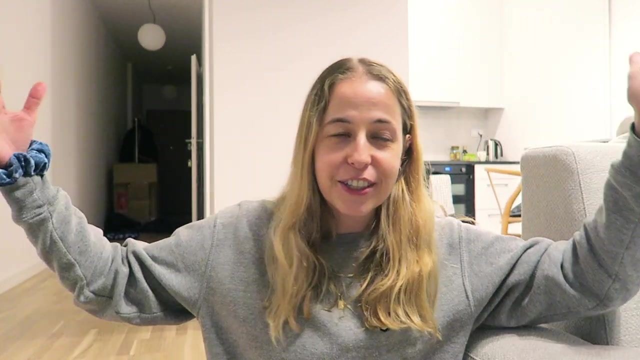 London, New York, right, finding a place to live in places like that it can be very difficult. in Copenhagen, even where I grew up, you don't choose a place, of course. now I'm kind of talking from a perspective of a young person. obviously, if you have the budget for you know, I guess, more expensive places and that's. 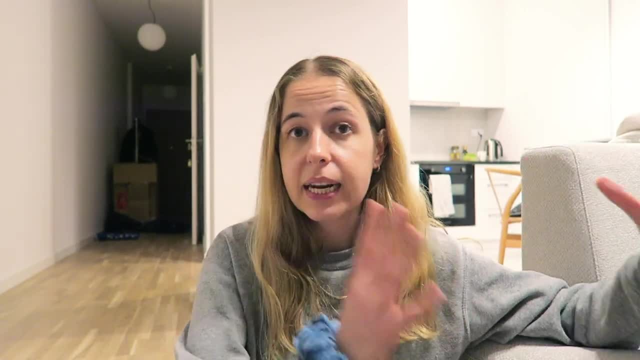 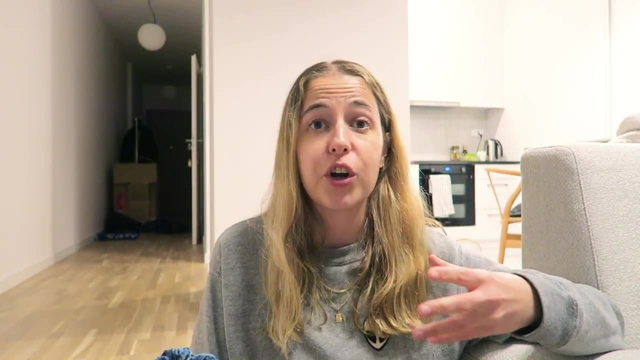 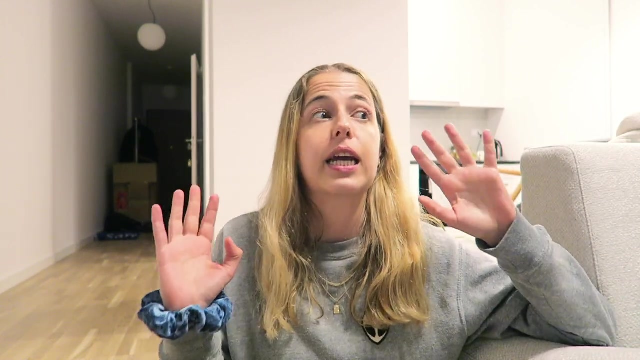 different story. finding a place to rent in many cities can be difficult, but in Warsaw it's not really a case. when I moved to Warsaw so it was like the first time in my life where I was actually like choosing apartments in a way both in like Shanghai and Paris. Paris is like- Oh- another story- Shanghai is not even. 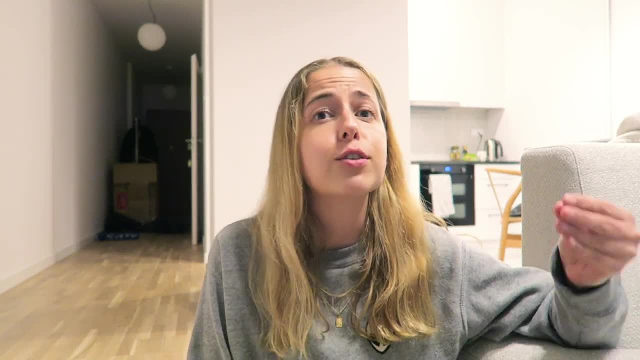 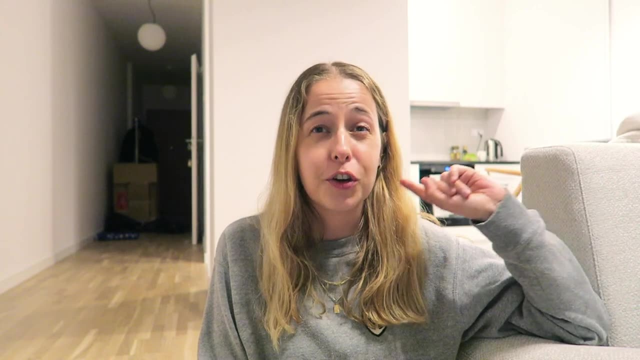 that bad, but, like Paris, is really bad. in Paris you don't choose you just you're happy if you get an apartment. that's the way it works in Paris and living conditions like that are just so important for you. but if you go to Japan are really bad as well in worse. it's not really the case, however. of course that 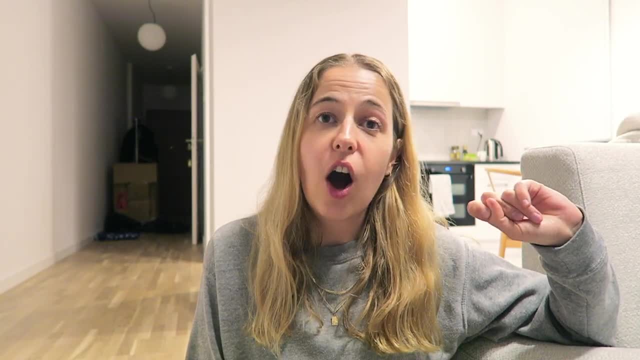 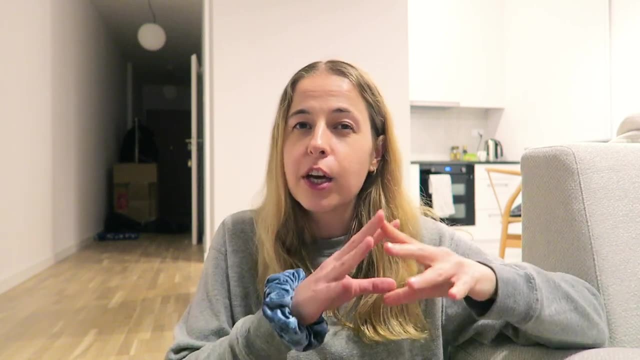 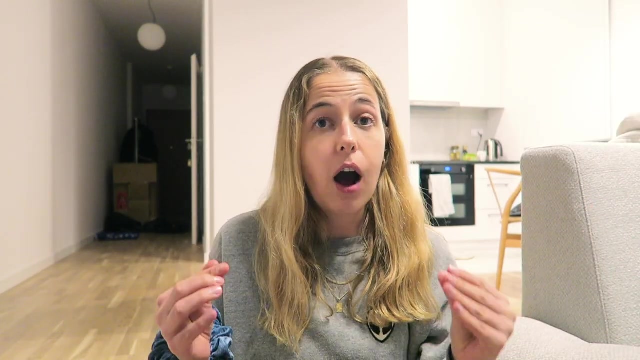 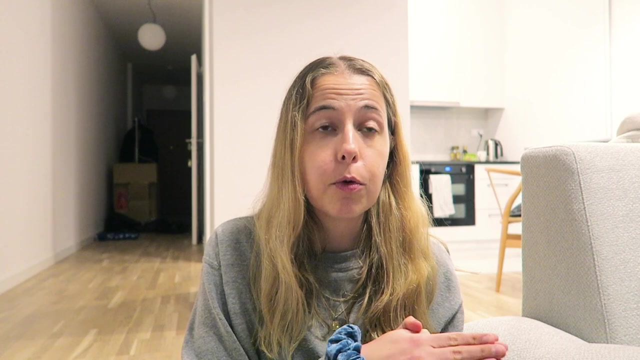 depends on your understanding of what good living conditions are. I would say that Warsaw, compared to other European cities, living conditions meaning that the size and standard of apartments is often quite good compared to many other big cities. in Warsaw, it is very much possible to be a 20-something year old. 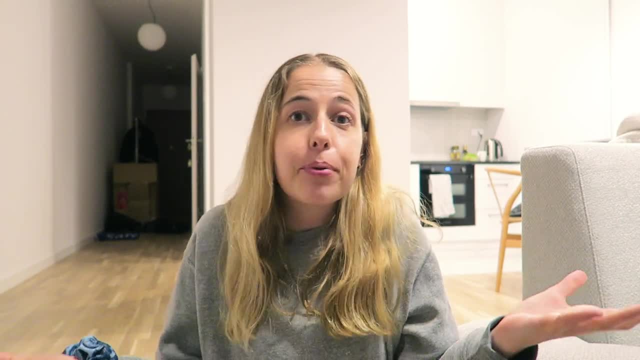 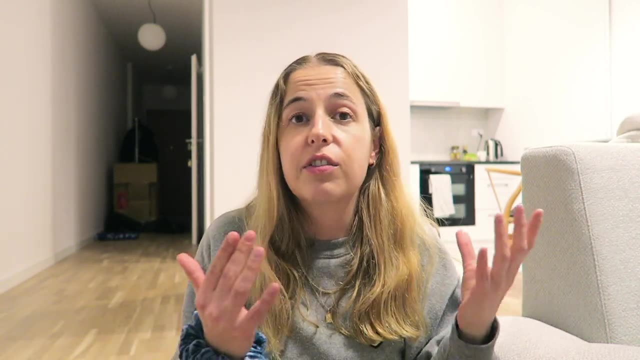 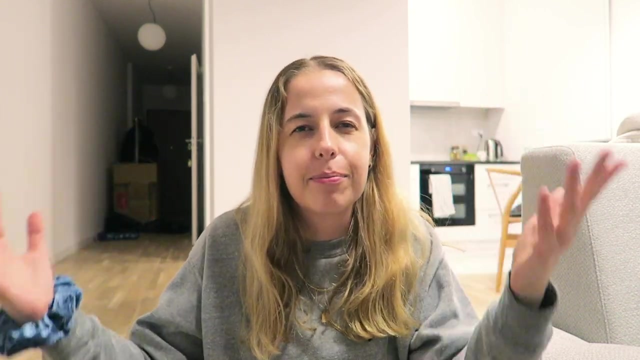 who just well, let's say, graduated and live in a pretty nice ish place where, for example in Paris, if you're a 20-something year old who just graduated, you're gonna live in a place that is extremely small and probably has a very little ugly kitchen and very little ugly bathroom. you get the point. 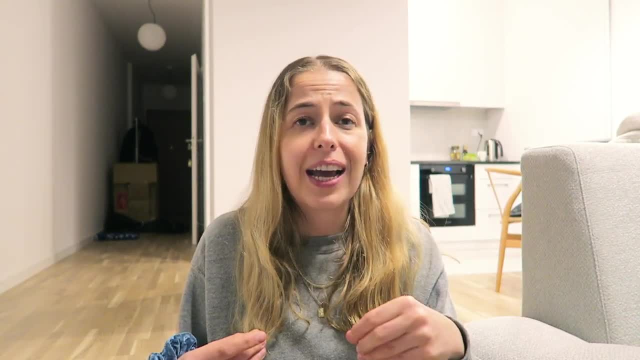 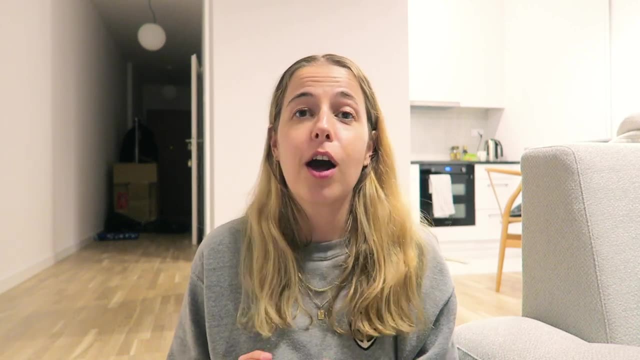 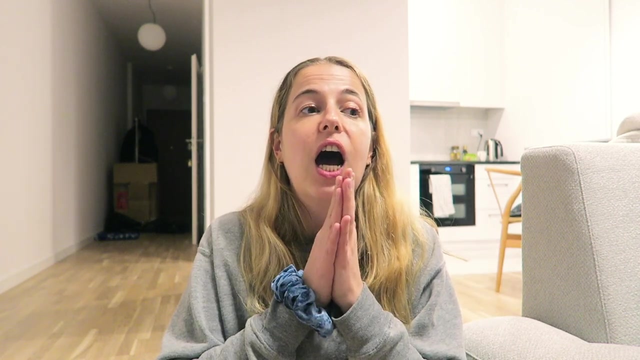 when I posted a video of my previous apartment tour, I did get some comments saying that my apartment was a little bit too small for me to live in. but I apartment was small and I was surprised by these comments because for me it was not small, it was like 40 square meters and I was the only person living there. 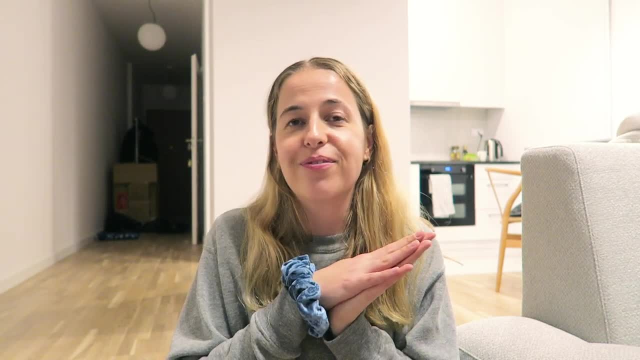 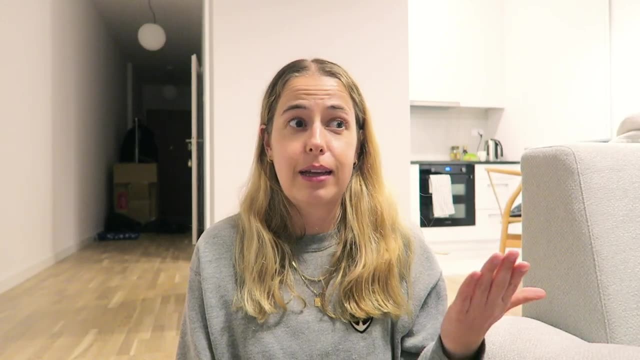 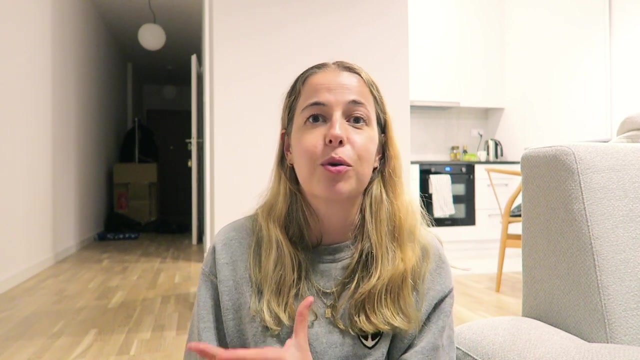 so, yeah, I was not gigantic, but I I would not need more. you know, for me it was like good enough, like it's actually like very good. to be honest, like I've lived in places that are much, much smaller- I obviously shared apartments with roommates in Paris- I've lived in a place that was like probably 17 square. 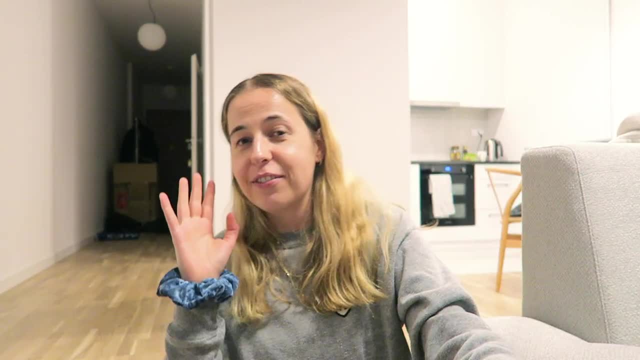 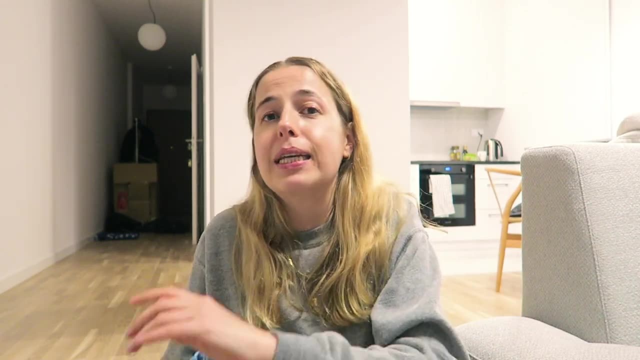 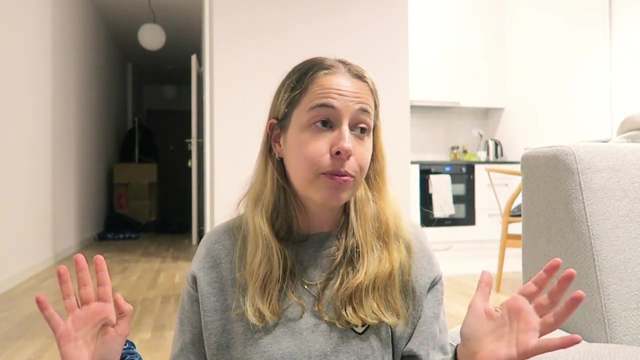 meters. so for me I was, like you know, luxury- 40 square meters only for myself. but I do understand that it really depends on where you come from. I know that in some places, like, let's say, in the States, people are used to having bigger spaces or whatever. so in general, in my opinion, living conditions in 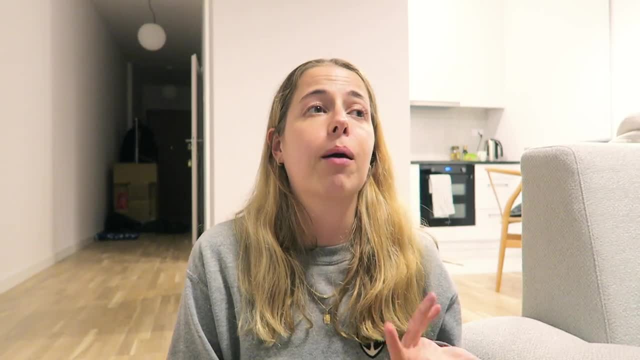 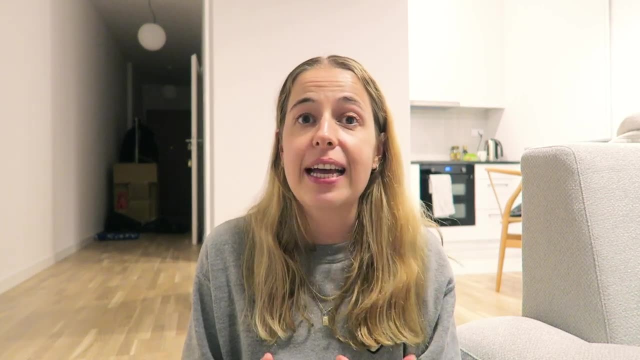 Poland are pretty good in that way and also the living conditions in Poland are pretty good in that way, and also the living conditions in Poland are pretty good in that way, and also the- the apartments like you can count on having little bit more like nicer living standards than many.